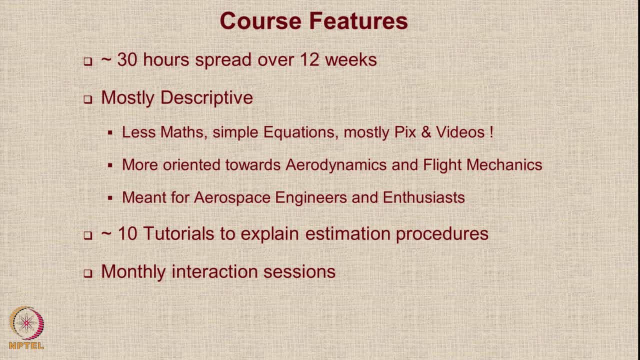 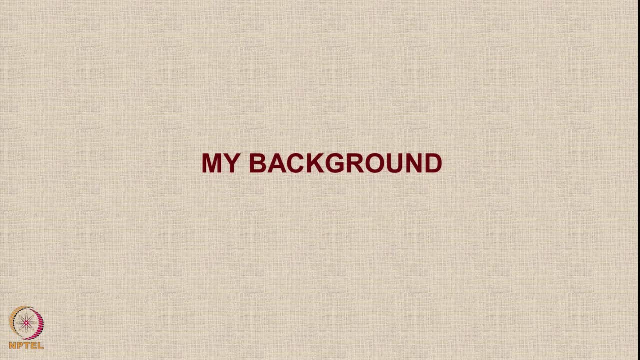 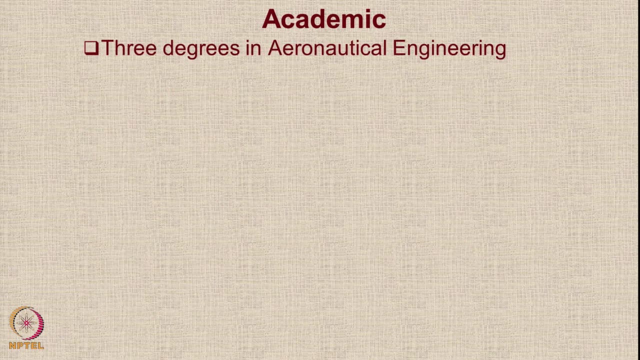 maybe more if needed, to clarify the doubts that you may have and also to explain some new concepts. Before I talk about the course, Let me give you a very brief idea about my background. On the academic front. I have 3 degrees in aeronautical engineering. The first of these, 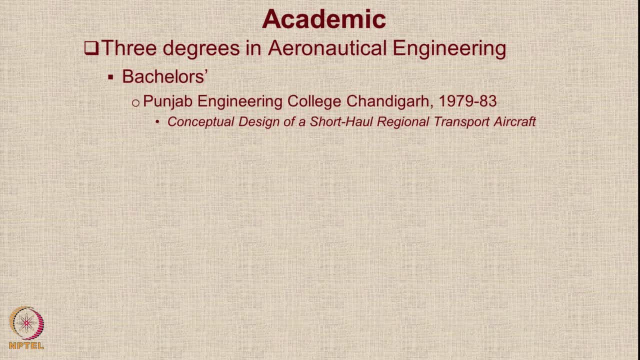 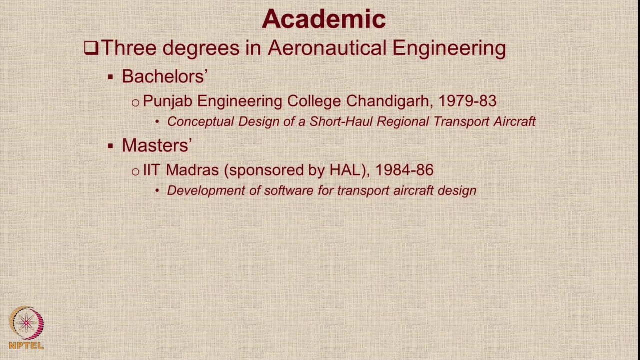 was the undergraduate degree Punjab Engineering College Chandigarh in 1983 and in my final year I lead a team of students who looked at conceptual design of a short haul regional business transport aircraft. Then I moved to IIT Mathras for his doctoral patt ice aircraft. 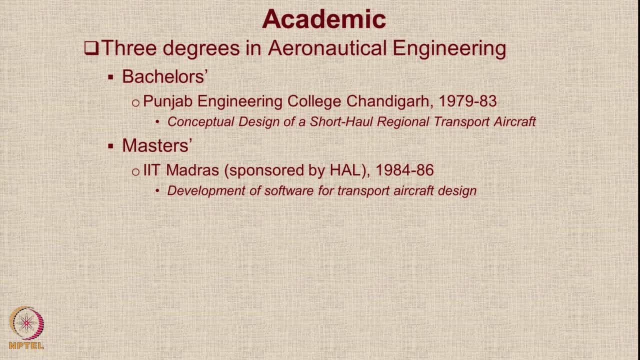 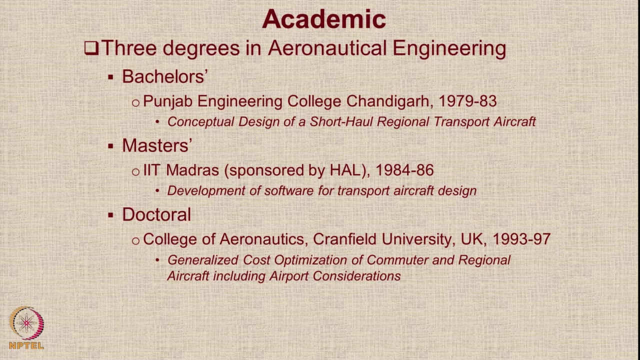 course 200.. master's program in aeronautical engineering sponsored by Hindustan Aeronautics Limited. As part of my MTech project, I developed some software for transport aircraft design. Subsequently, I went for a PhD at Cranfield University in the College of Aeronautics. 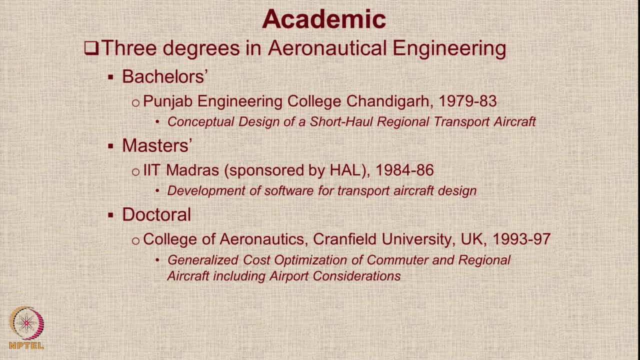 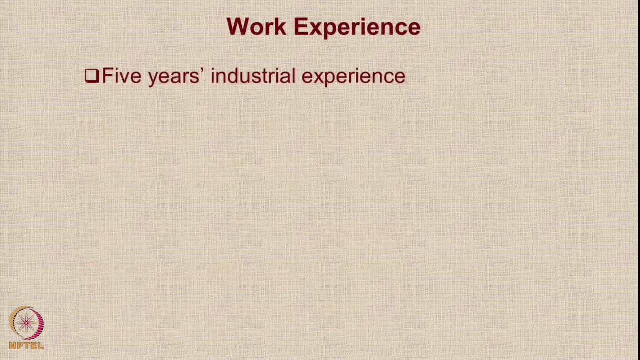 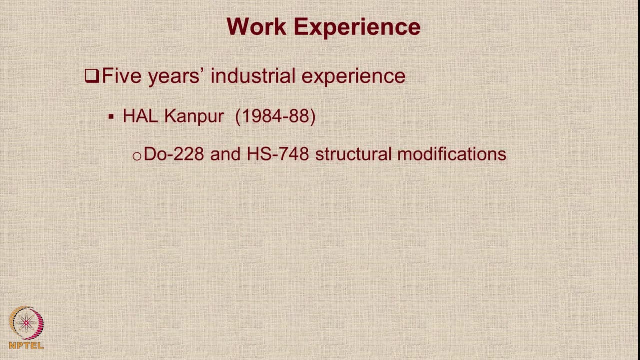 and my PhD thesis also is related to a topic in aircraft: conceptual design. As far as my work experience is concerned, I have five years industrial experience in Hindustan Aeronautics Limited in the design and development division, Of which the first three and a half. 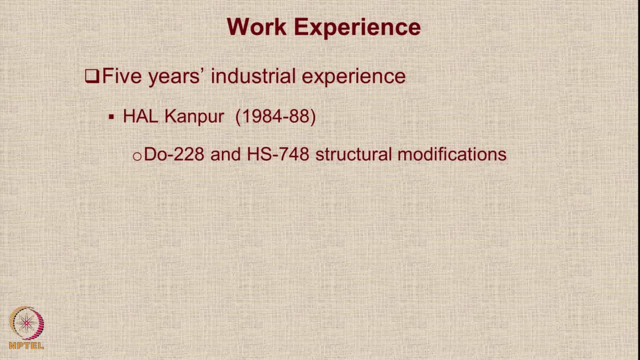 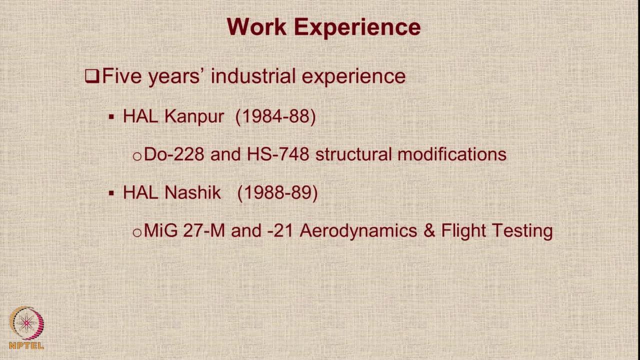 years were spent in HAL Kanpur, from 84 to 88, in which I worked on the structural aspects, and then I was promoted and transferred to HAL Nasik, where I spent one and a half years. There I shifted to aerodynamics and flight engineering. 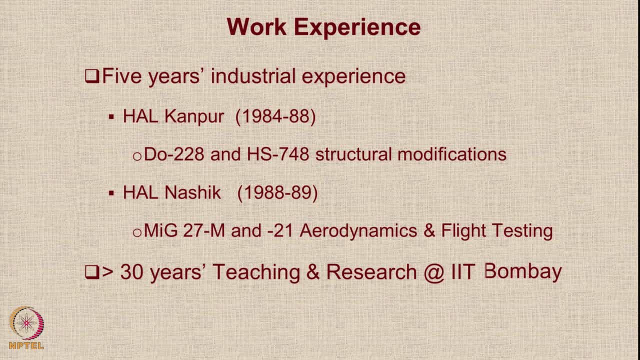 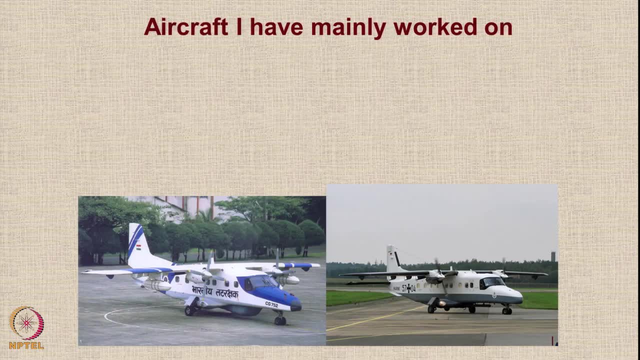 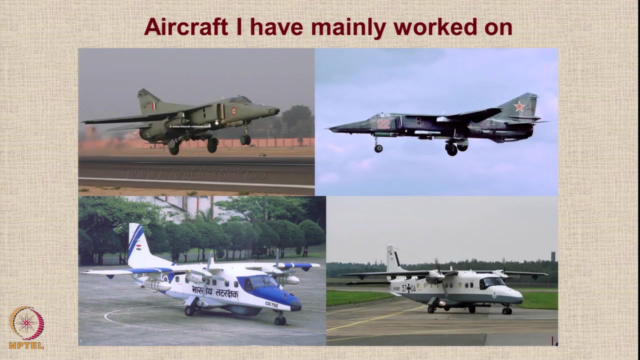 testing. After that I moved to academics at IIT Bombay, where I have spent around 3 decades. These are the aircraft on which I have mainly worked on when I was in HAL. The ones that you see on the bottom is Dornier DO22A-212.. And then, when I shifted to NASIC, I spent most of my time. 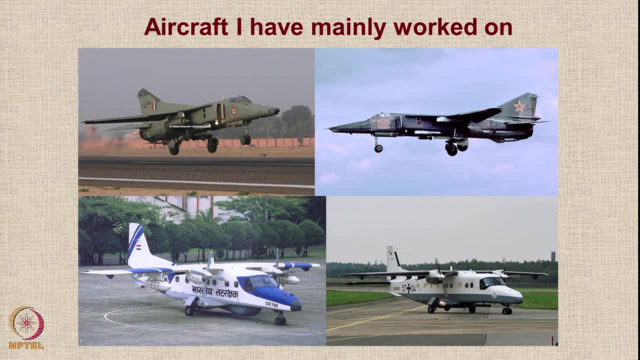 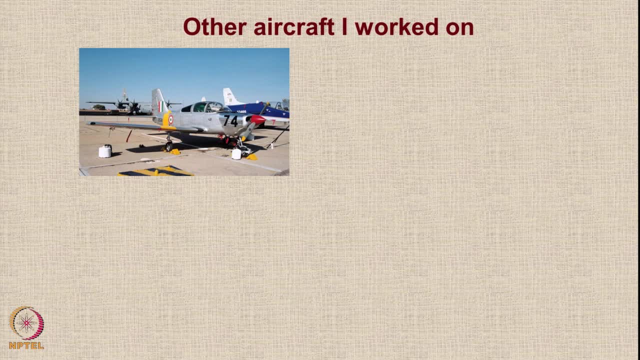 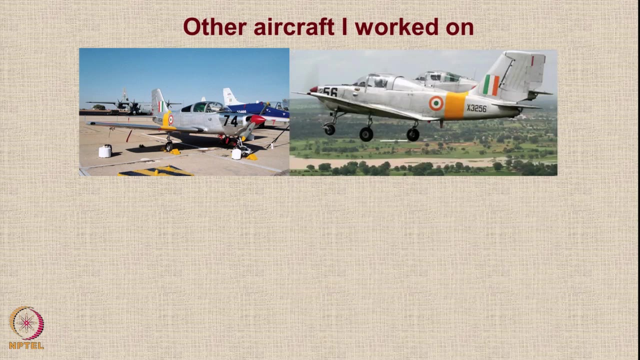 working on MiG-27M Bahadur aircraft, which at that time was being produced under license. There are some other aircraft on which I have worked. This is the HTT-32 aircraft designed by Indian design engineers of HAL Bangalore. It was then converted into a turboprop version called